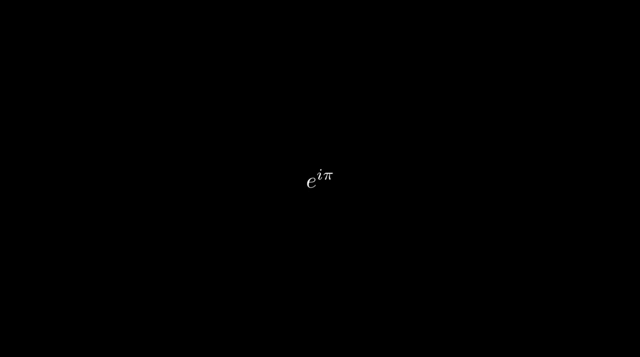 Consider a set of finitely many elements. We call the number of elements of the set as cardinality, and the number we get is called a cardinal number. It's therefore an easy task to find the cardinality of a finite set. However, things get interesting once we start. 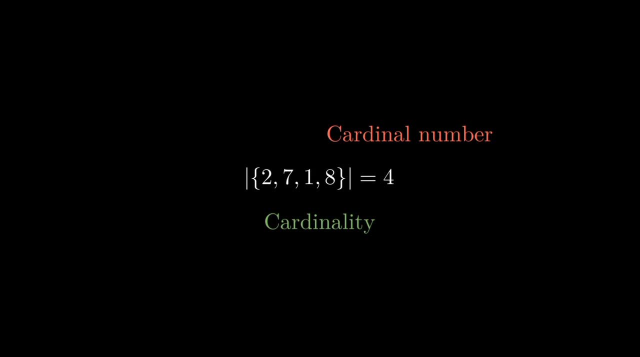 dealing with the infinite sets and, just as a side note, the term cardinal numbers are still valid even for infinite sets. For instance, consider the set of all natural numbers. Clearly it has infinitely many elements. Let's denote its cardinality by this stylish 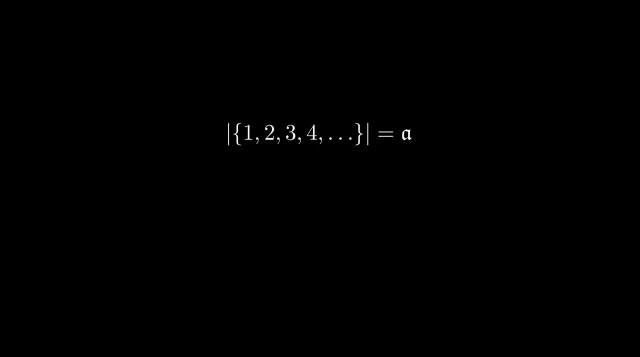 a. Now let's consider the cardinality of real numbers Again. it contains infinitely many elements, but is its cardinality equal to a In the language of notations? if the cardinality of this set of real numbers is c, are these: 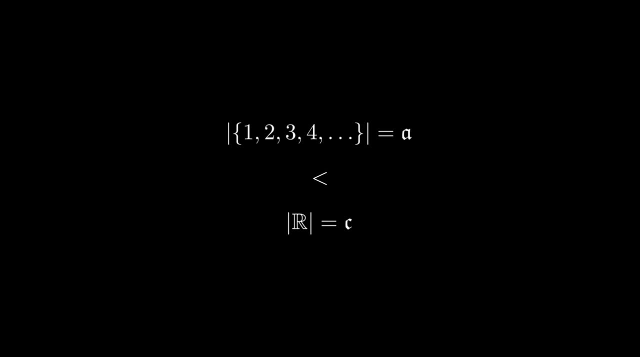 two equal Well? Cantor proved that they are not. In fact, c is greater than a And, interestingly, it's this. This means that there are further classifications of infinite and that some infinites are larger than the others, Like in this case. we can conclude that the number 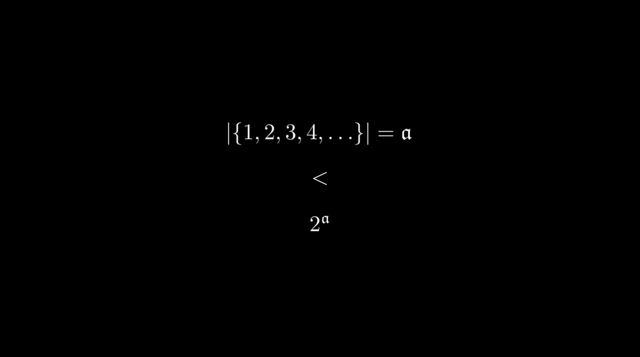 of real numbers are more numerous than the natural numbers In general. if we have a set and if we can establish a bijection between the set and the set of natural numbers, then we call that set countably infinite And notationally we call its cardinality a. We note that it's not possible to establish a bijection. 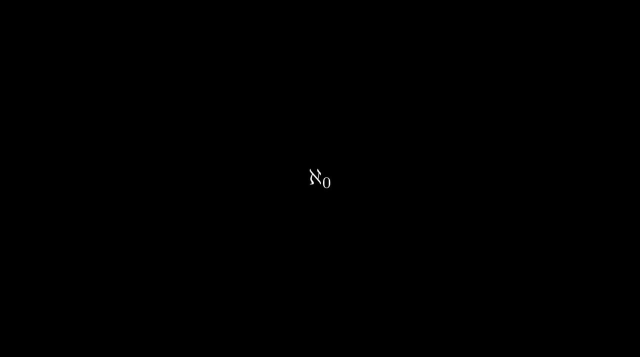 between the real numbers and the natural numbers. Hence, the set of real numbers is uncountably infinite. In fact, its cardinality is equal to the cardinality of the power set of the naturals. Using the previous expressions we encountered, we therefore have c equals 2. 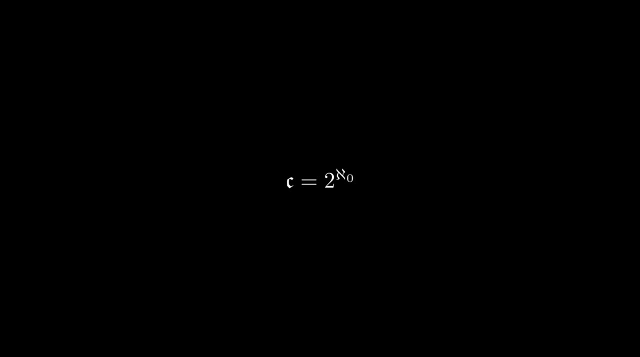 to the power of a. Another important notation that we must care about is Lf1.. In extreme simple words, it's the cardinal number, which is just greater than Lf0.. In other words, there aren't any cardinal numbers between Lf0 and Lf1. 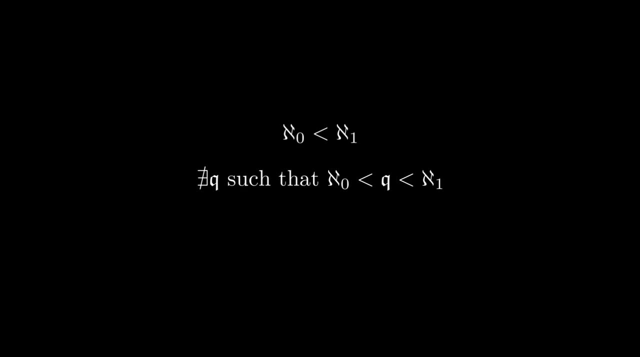 Let's now have a glimpse of the problem whose proof was tried by Cantor for quite some time: the continuum hypothesis, The statement of continuum hypothesis, says that we can't find a set whose cardinality is between Lf0 and 2 to the power of Lf0. In other words, 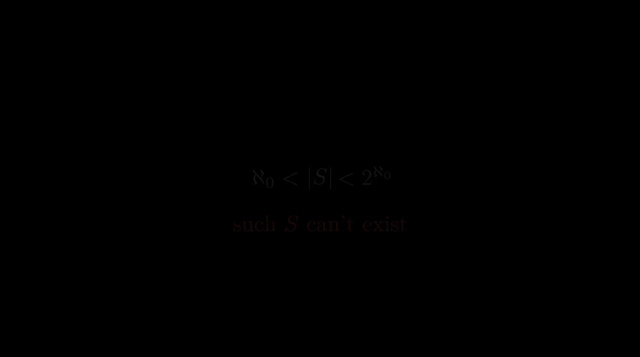 Lf1 equals 2 to the power of Lf0.. Also the first of Hilbert's 23 problems, it's a source of numerous debates among mathematicians. A more general statement of continuum hypothesis says that if the cardinality of an infinite 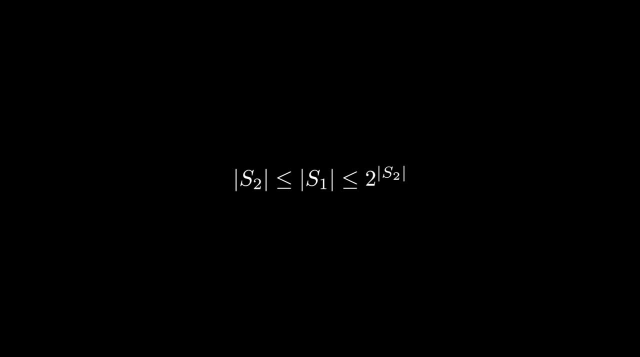 set lies between the cardinality of another infinite set and the cardinality of its power set, then the cardinality of the set is either 0 or 0.. It's interesting enough to know that the continuum hypothesis is independent from Zermüller-Fraenkel set theory. Gödel showed that the hypothesis can't be disproven from. 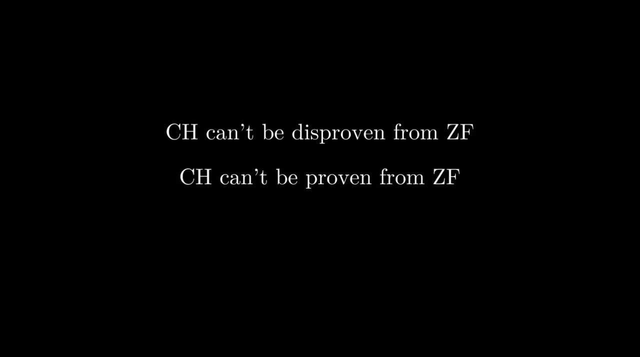 Zf. On the other hand, Cohen showed that it can't be proven from Zf. Therefore, it became clear that continuum hypothesis is independent of Zf. Gödel believed that the continuum hypothesis is independent of Zf. Gödel believed that. 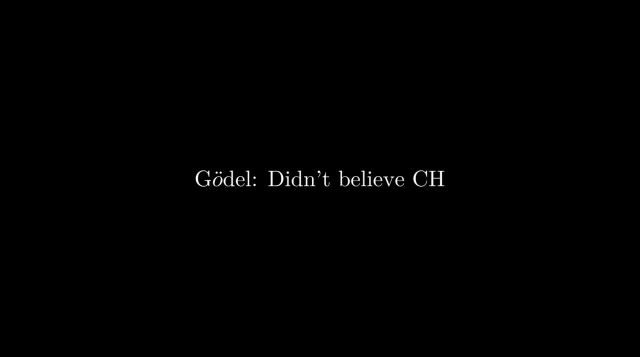 Zf is consistent with Zf. The hypothesis is false, even though he had shown that the hypothesis is consistent with Zf. This interestingly implies that Zf-exe jumps aren't enough for the universe of sets. Even Cohen believed the falsehood of C? h. 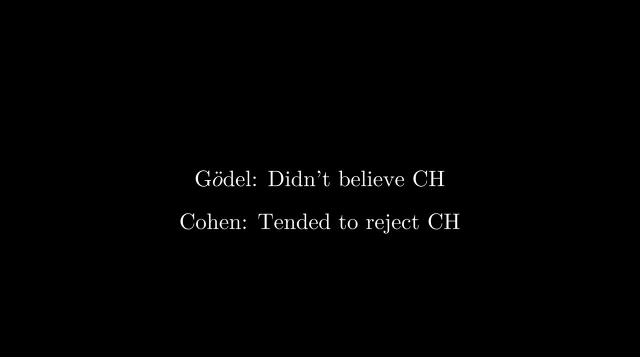 An interesting viewpoint is that our conception of the set is not specific enough to conclude the correctness of C h- Skolem had argued on the same- on the basis of a paradoxical statement where, from a countable model of ZF axioms, we are able to take an uncountable set. 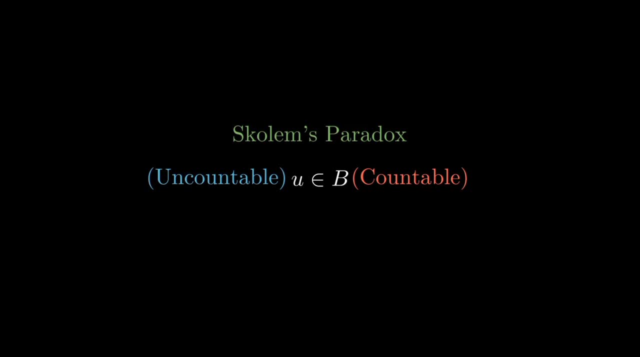 The argument was supported by the independence of CH from ZF. To get against the idea we can demonstrate new axioms to resolve CH in some direction. Some interesting stuffs are associated with the arguments of W Hugh Woodin where he gave the concept of star axioms, which implies that refrigerator is LF2.